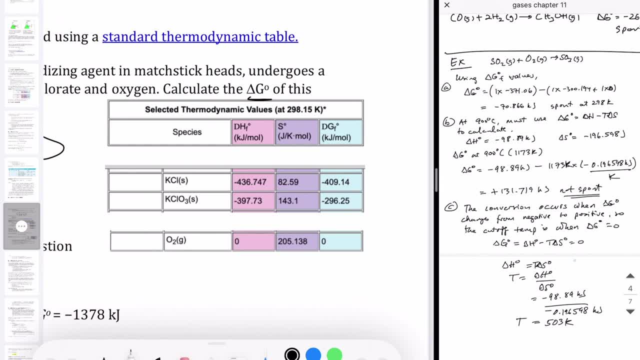 several reactions to manipulate. So I've gone into our thermodynamic table to pick out exactly the numbers that we are going to need. So if you're going to use your delta H minus T, delta S formula, then you're going to need to use these thermodynamic values to calculate. 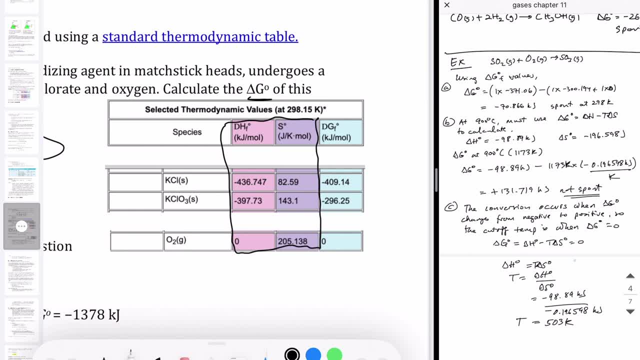 the delta H and then the delta S and then like this: Lastly, apply it to that formula. If you're going to use your formation values, all you need is this blue column right here and then just subtract the products minus the reactant. 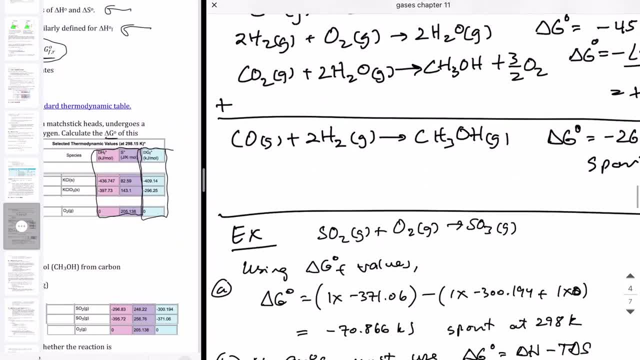 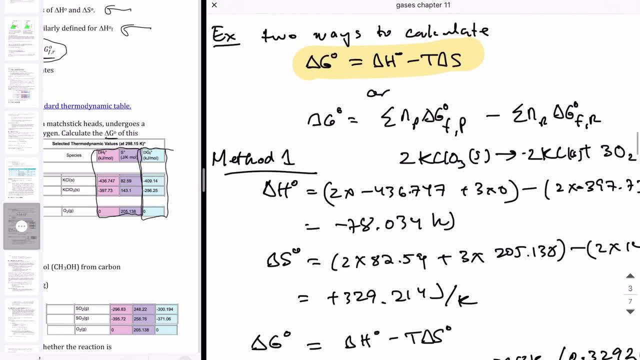 and you'll get your number. So I will do it both ways to show you that both methods give us the same conclusion in the end. So in method one, all I'm going to do is using this approach. So that means I have to calculate my delta H, which I can do by taking products minus. 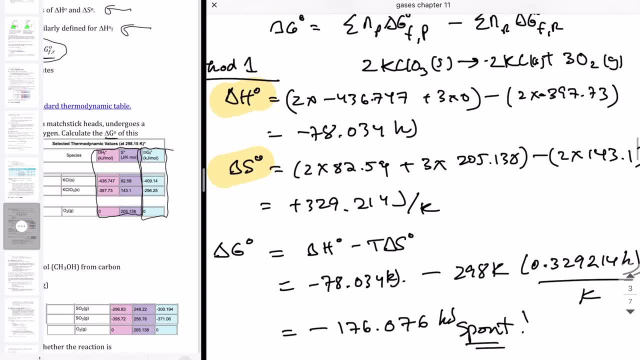 reactant of the formation, enthalpy, and then I can calculate my delta S. In this case I'm taking the molar enthalpy, So I get this for delta H and that number for delta S. I always want to remind people. 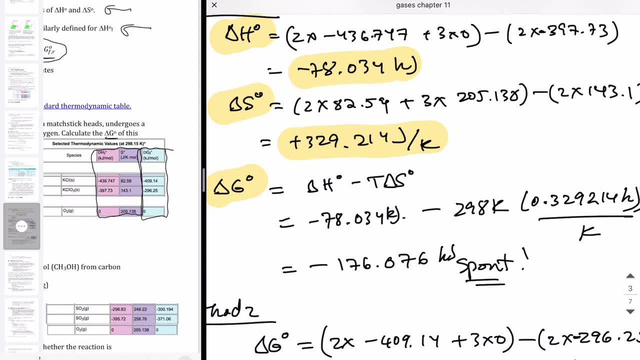 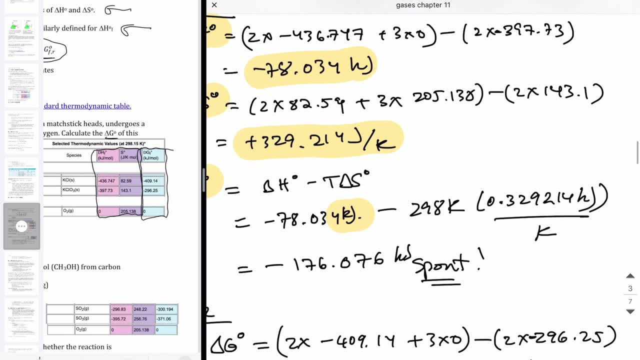 that the units are different for the two quantities. So when you bring them to calculate delta G you want to make sure that you put them on the same unit. So here I put both of them in the kilojoules unit. So I keep the delta H the same, but then the delta S I changed. 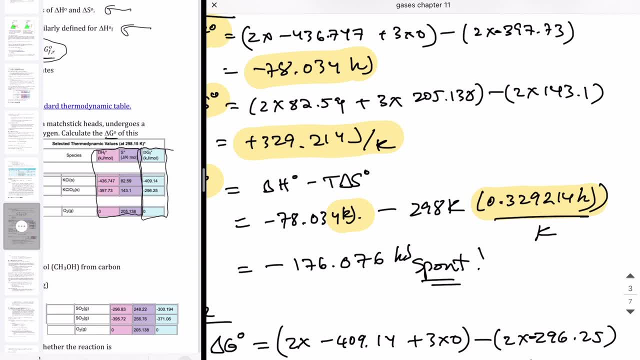 it to kilojoules with. dividing it by a thousand make it 0.9214 kilojoules per Kelvin, And when I multiply it by 298 Kelvin, I get 0.9214 kilojoules per Kelvin. And when I multiply. 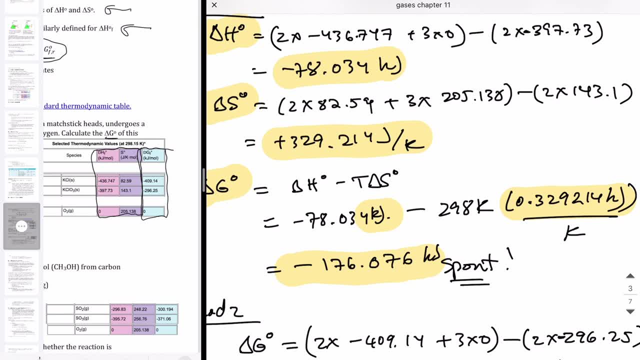 it by 298 Kelvin, I get 0.9214 kilojoules per Kelvin. And when I multiply it by 298 Kelvin, I end up getting this value negative 176 kilojoules, which tells me that my reaction. 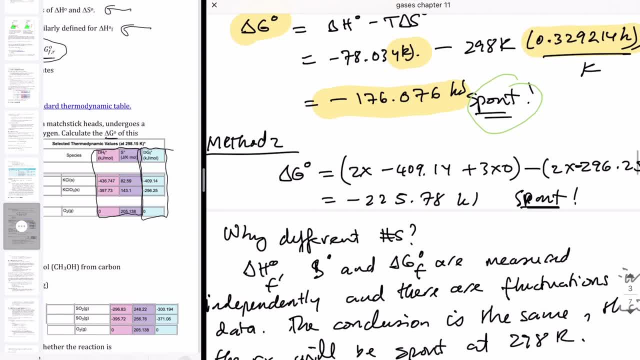 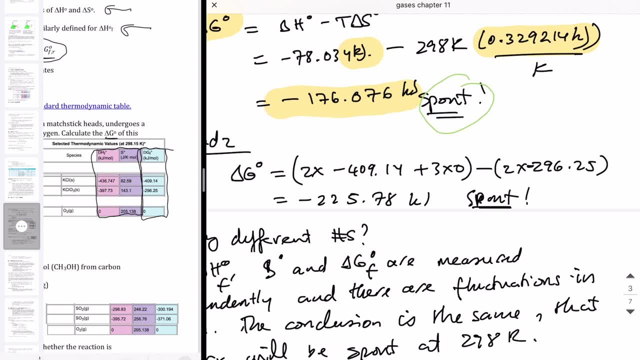 is spontaneous, because I have a negative delta G. Now what about the second method? The second method uses that Gibbs, free energy of formation, And in that case I just plug in the number I have given in that thermodynamic table. I ended up getting negative 225.78 kilojoules. Now this is a negative number, So it tells. 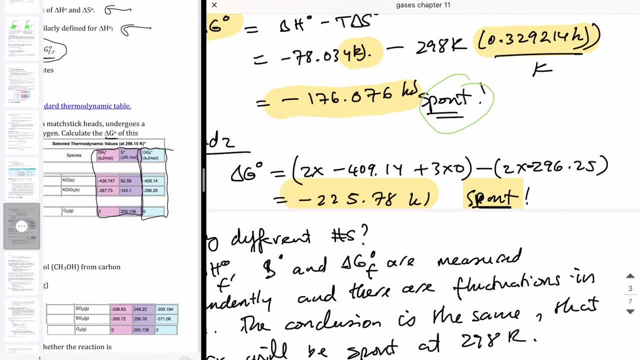 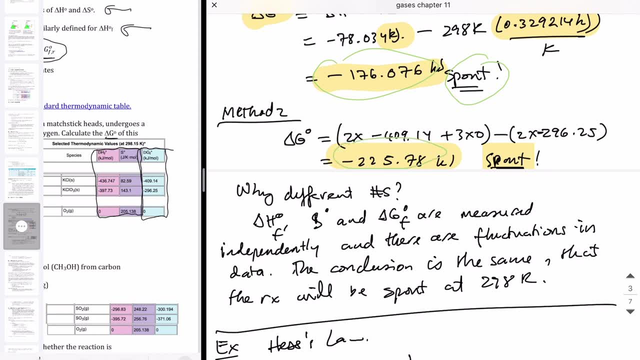 me that the reaction is spontaneous. So in both ways I found that my reaction is going to be spontaneous. The immediate question that you might have is: why do we get different numbers? Here we got negative 176, here we got negative 225.. The reason, primarily, is because the delta. 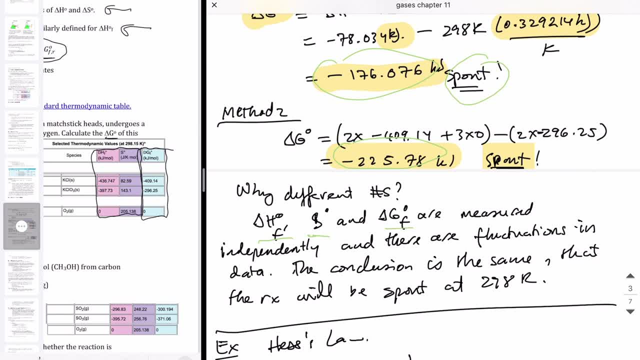 HF, the molar entropy and then delta G formation are all measured independently of each other. So there is some fluctuation in the measurements of these numbers. But the key point to take home here is that both calculations tell us that the reaction is going to be spontaneous. 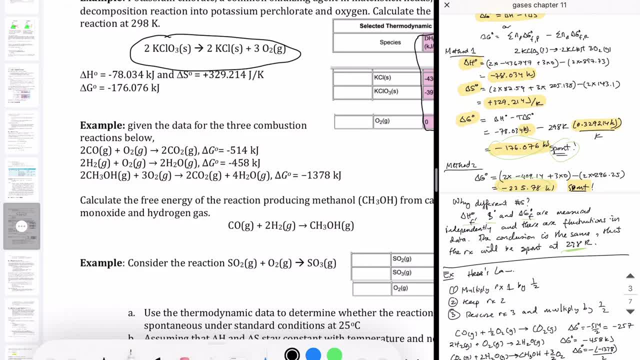 at 298 Kelvin. Now let's take a look at the second example. So this is a reaction that we're given in your lecture notes, And here we see that we're given a series of reactions. All of these are combustion reactions And we were told 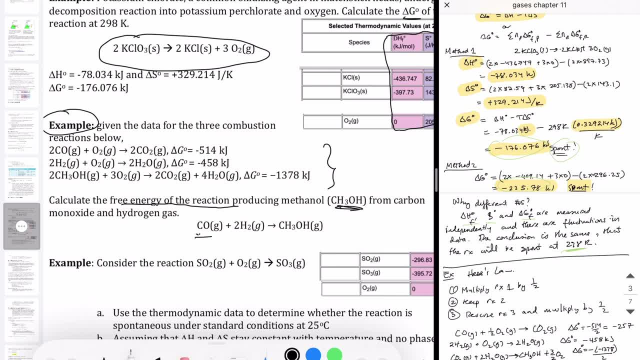 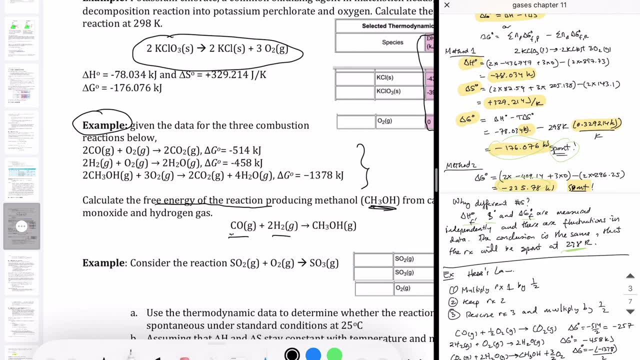 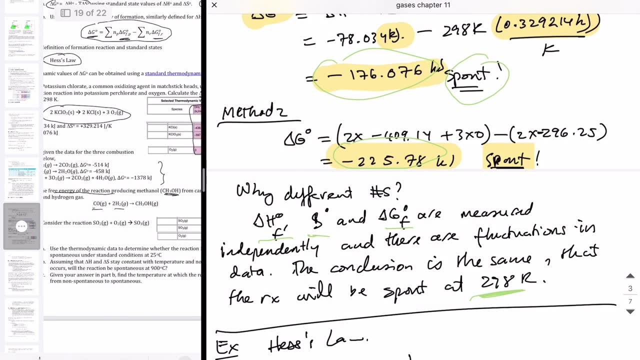 to calculate the free energy for the reaction where methanol is produced from carbon monoxide and hydrogen gas. And so when you look at a question like this, the thing that should immediately jump up at you is the fact that we have few reactions. We can manipulate this reaction, So that means 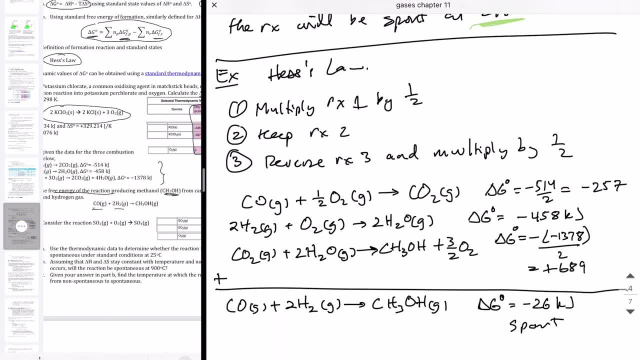 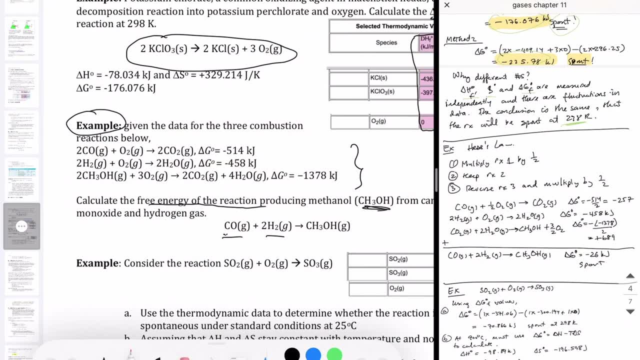 Hess's law Right, So we're going to work on that. So what I want to do with Hess's law is always to take a look at all the reactions that you've given and see how you can get to the final reaction. The way I do this is: I try to circle. 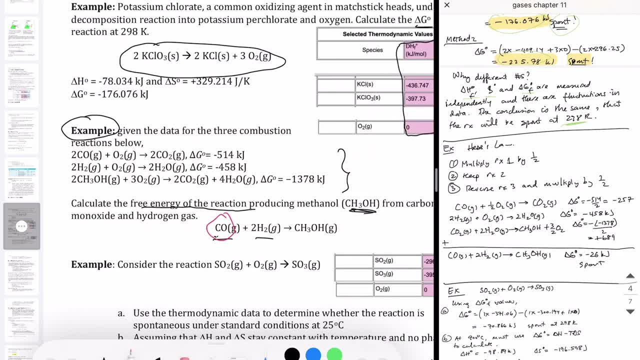 the species that I need at the end. So I need a CO gas in my reactant. So I look at all my three reactions. I notice that there's a CO right there, but it's two. So that's something I need to work on. And then I need a 2H2 also in the reactant. I have a 2H2 on. 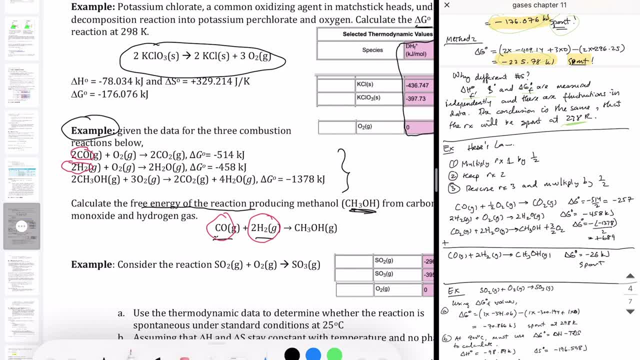 that second reaction and nowhere else Right. So that means that I need something to keep that. And then, lastly, I need my methanol CH3OH in the product with the coefficient of one. I have a CH3OH right now on the reactant. 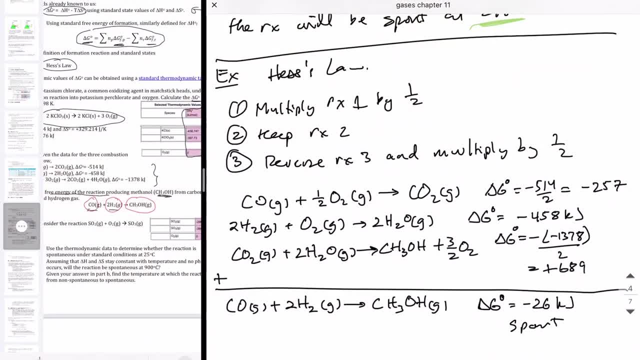 my reaction three. So I need to do something with that. And so, given the setups of what I want in my target reaction, I'm going to need to multiply reaction one by a half. that would make my two carbon monoxide become one carbon monoxide. I need to keep reaction two. 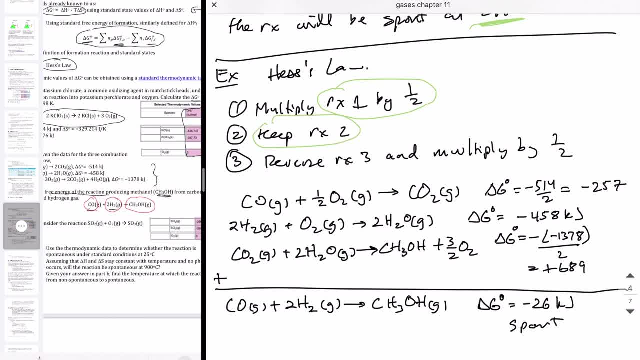 as is, because I already have two H2 there, So I don't need to change anything, And then I need to reverse reaction. three, because my methanol is given as a reactant, but I want it in the product side, And I also 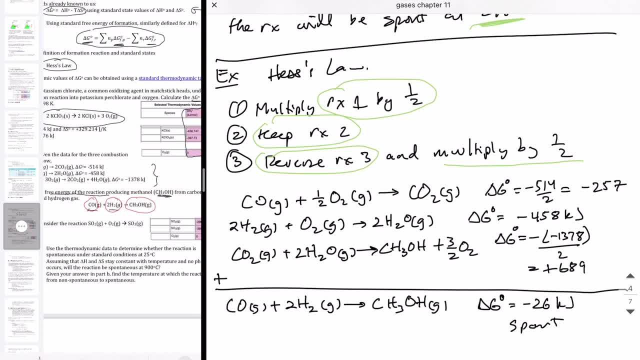 need to multiply it by a half because in the given reaction, my methanol has a coefficient of two. My target reaction, my methanol, has a coefficient of one. So those are the three things that I need to do to my three reactions. So these three equations here are the reactions. 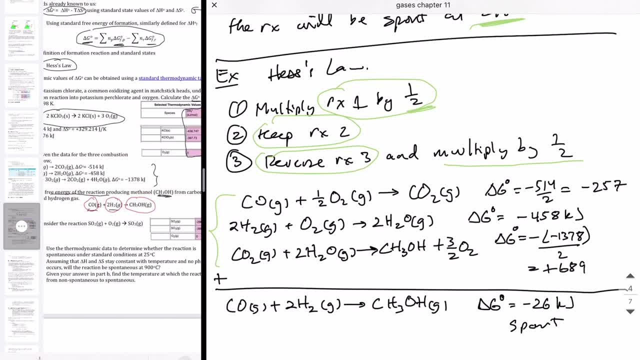 after I've done all those three things to it. Now you remember that if you were to multiply something by a half, that means you're going to multiply that Delta G value by a half as well, which gives negative 257 kilojoules. I'm not writing the unit here just because 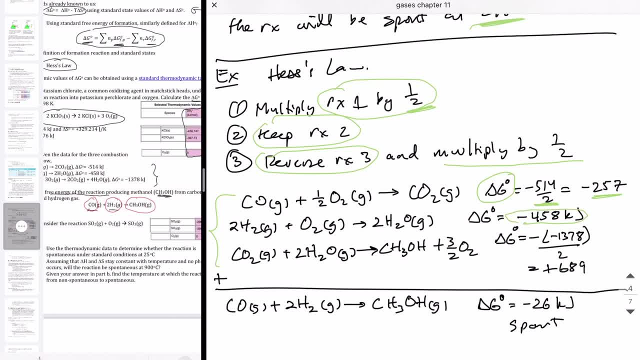 of space constraint. The reaction two was unchanged. So the Delta G is the same, which is negative 458 kilojoules. And then the last one: I reverse the reaction, which means now the Delta G is the negative of whatever the original value is. The original value is negative. 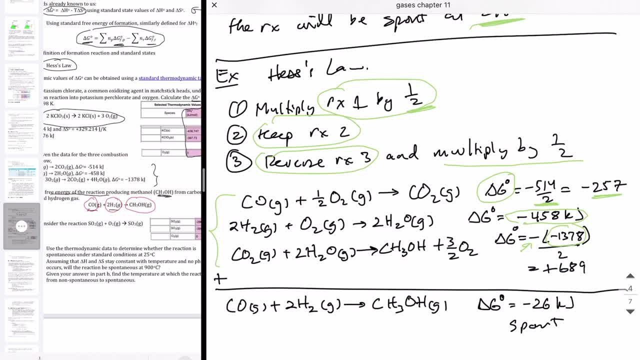 1378.. So it's negative of that number And then, since I multiply it by a half, I divide it by here as well, which gives me a total of positive 680 for that reaction. And then what I need to do now is add all the numbers that I have and then see if I get the total reaction that 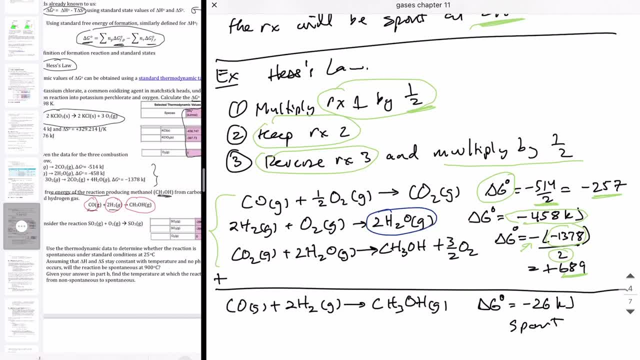 I want or not. So you notice that a few things cancel out. so the 2H2O are the same and then one is on the reactant, one is on the product, So they cancel. I have three halves O2, 1.5. 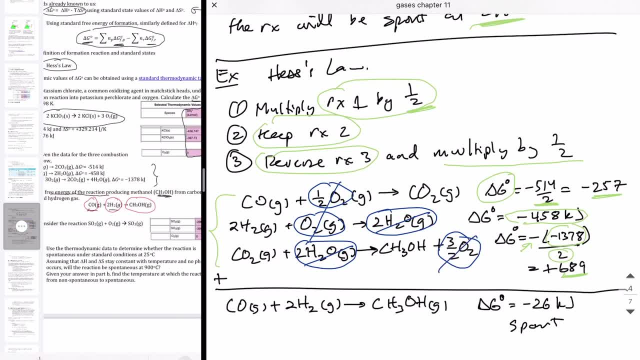 O2.. I have a half, I have one, So those cancel out as well. And then I have a CO2 gas on opposite sides. well, so what i have in the end is co2h2 on the reactant side and methanol on the product side. 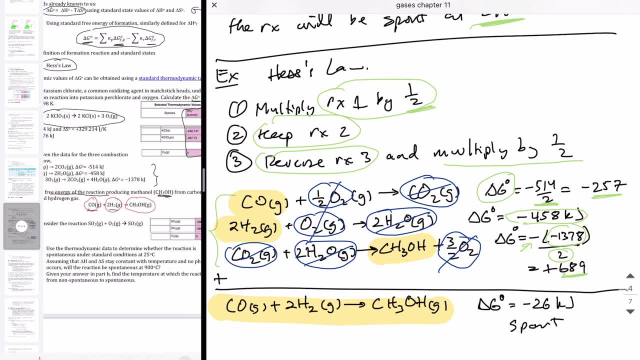 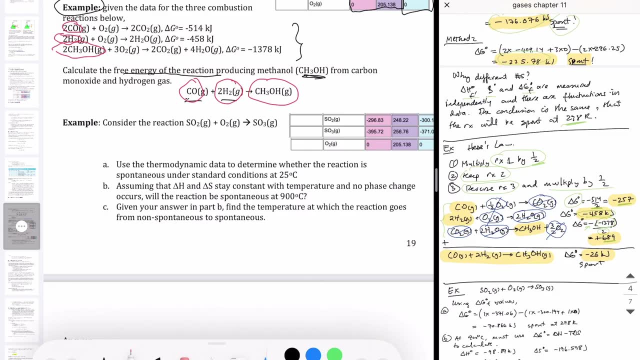 which is this thing and that's exactly what i want. so into to get my delta g, i just need to add these three numbers: the negative 257, the negative 458 and then the positive 689. that gives me negative 26, which tells me that this is spontaneous. let's now take a look at the last example on the 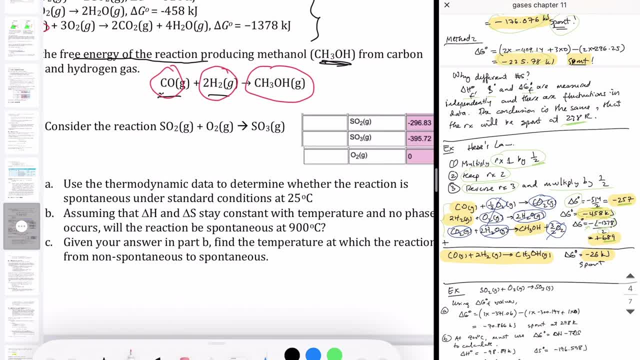 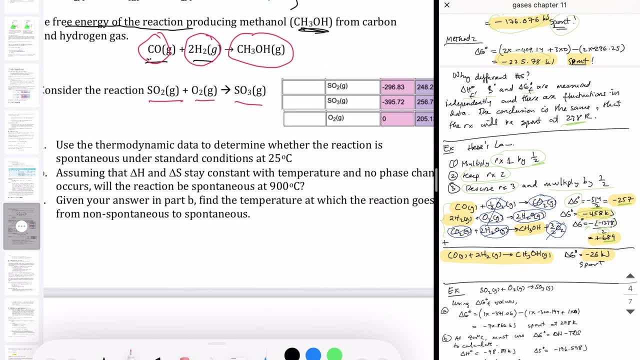 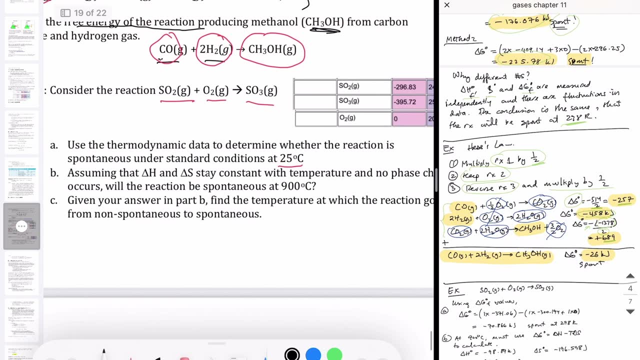 calculation of delta g. so now we're given the reaction so2 and o2 going to so3, and we're asked a few questions about it. the first one is to just use the thermodynamic data to determine whether the reaction is spontaneous under standard condition at 25 degrees celsius and then in the 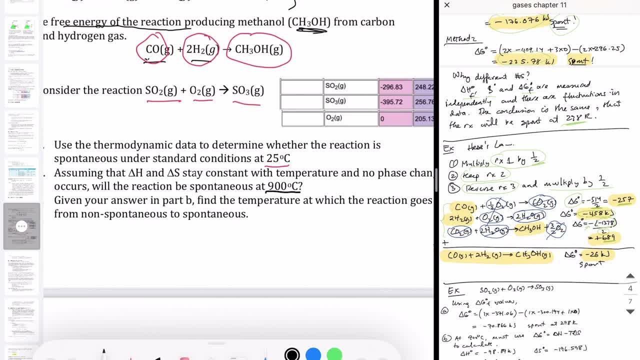 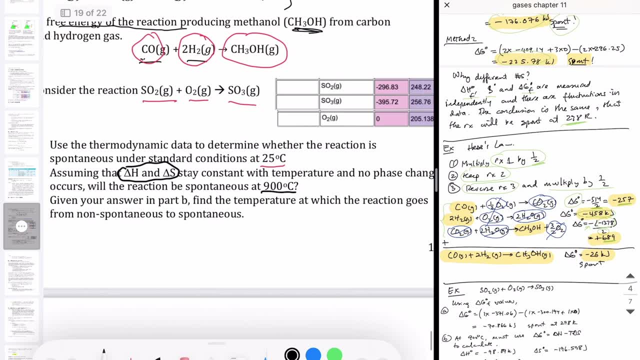 second one: we were asked if that reaction is still going to be spontaneous at 900 celsius, and here we're told to assume that delta h and delta s values stay constant with temperature. and then the last one is: we're asked: what is the temperature at which the reaction goes from non-spontaneous? 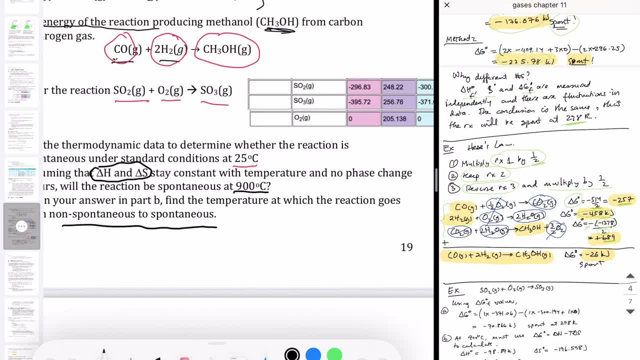 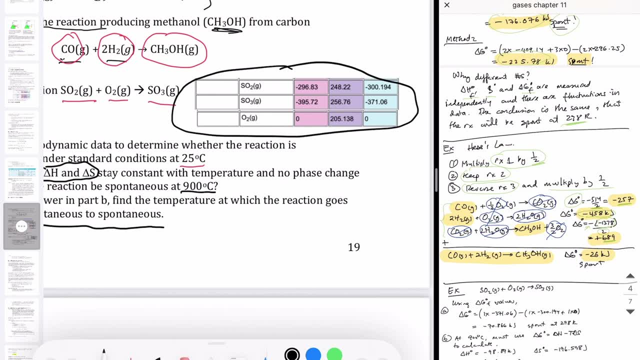 to spontaneous. okay, so we're going to have to calculate a value of temperature there. let's start with part one a. all you need to do is just take a look at your thermodynamic values, which again i've copied just the relevant parts here from that table, and remember that the last 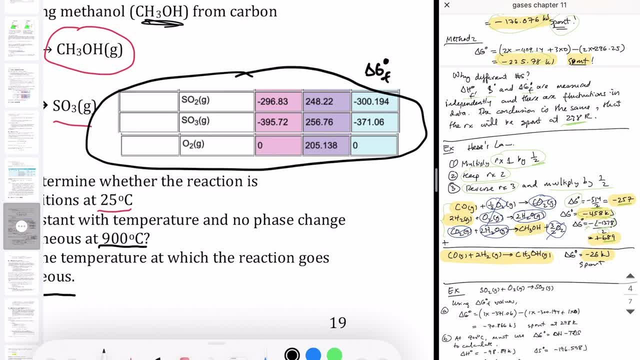 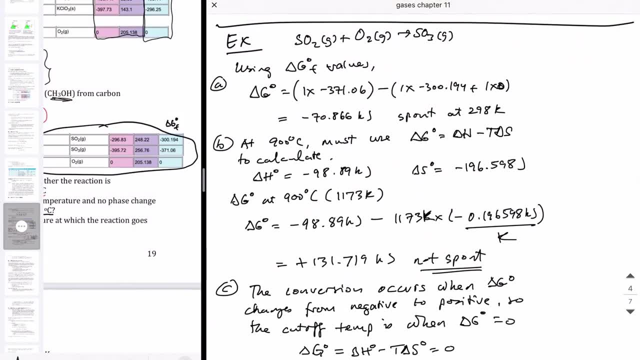 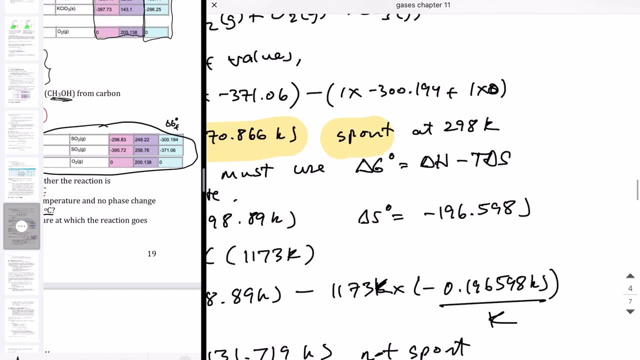 column here is the delta g formation value. so i'm just going to use that to make my calculation, because that's the shortest way to get to my delta g value. so let me show you what that number is once i calculate it, and that ends up being negative 70.866 kilojoule, which tells me that 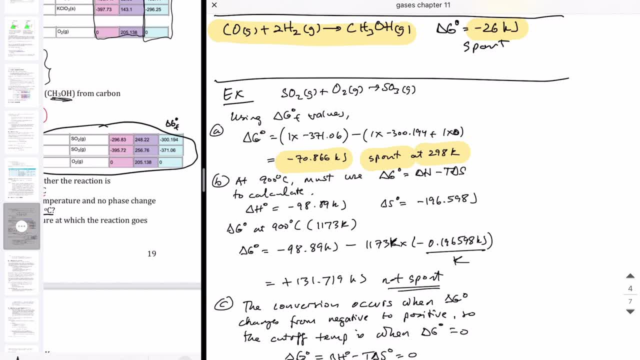 the reaction is spontaneous at 298 kelvin. but you will see that a lot of times this calculation that's done using the formation delta g is for 298 kelvin, because that's where those values were measured, at 298 kelvin. so just keep in mind that when you're trying to 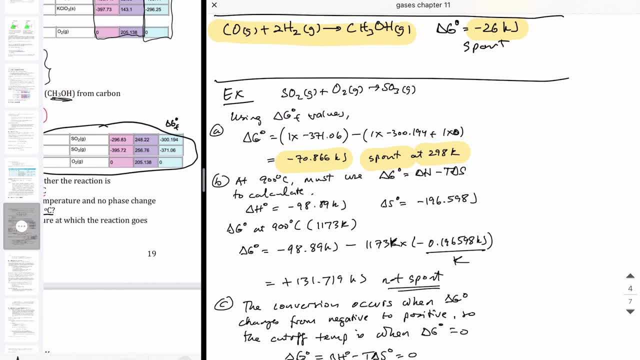 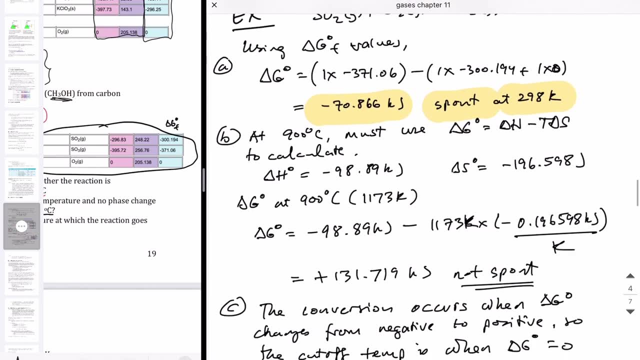 calculate at another temperature. you can't really use that number. if you're using that number, you're making the assumption that the value of delta g doesn't change with temperature, which is incorrect because we know it does right and in fact that's what question b is asking. it's: 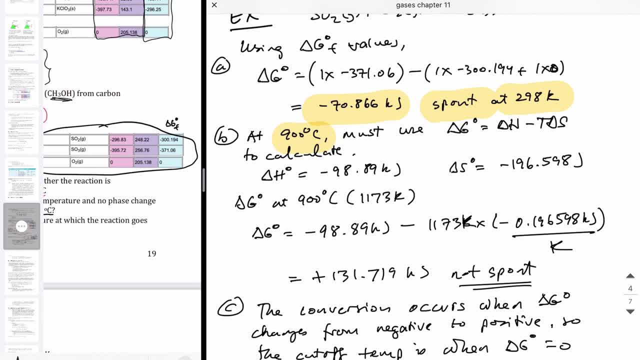 saying, at 900 celsius what is the value of delta g and is the reaction spontaneous or not? this is important because now you can't just look at the same number that you calculate and say, okay, well, it's negative 70.866, so it's going to be spontaneous, because that only applies to 298. 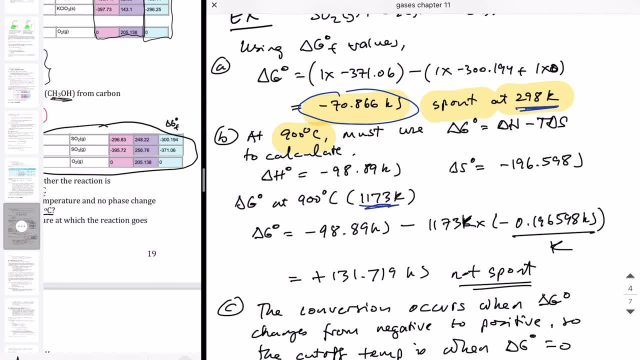 kelvin. if you're going to calculate it at 900 celsius or 1173 kelvin, you're going to have to use this equation, which is: the delta g standard equals to delta h standard minus t, delta s standard. right, so you're going to have to use that equation, because that equation explicitly has a. 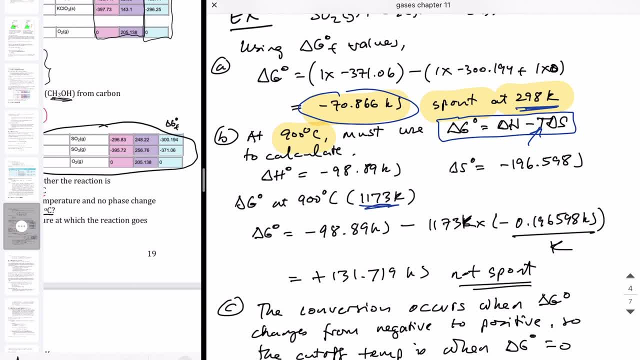 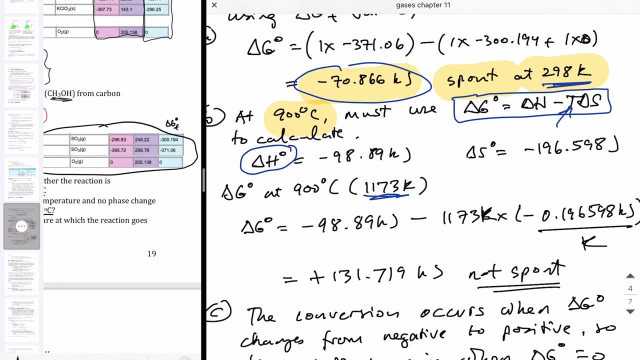 temperature factor here which is going to give us a different delta g value. so for this i'm going to have to go back to my thermodynamic table and find the delta h standard. i can use the formula of formation intel, which is product minus reactant, to calculate it, and when i calculated it i get. 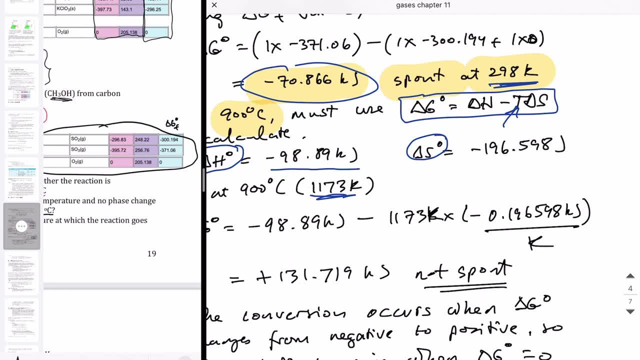 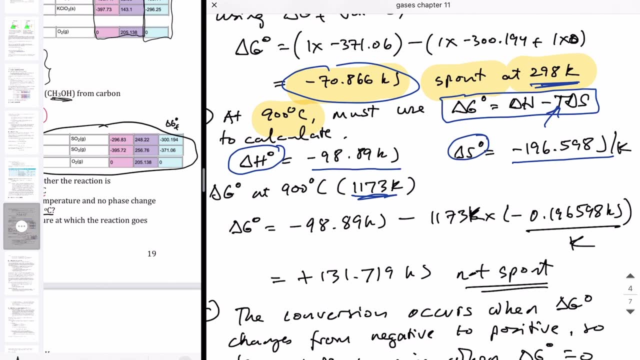 negative 98.89 kilojoules for the delta s standard. i can use my molar entropy values again from that thermodynamic table, and i found that the number is negative 196.598 joules per kelvin. okay, so remember that that's the unit of entropy, and now i'm going to put it together to calculate delta g at 900. 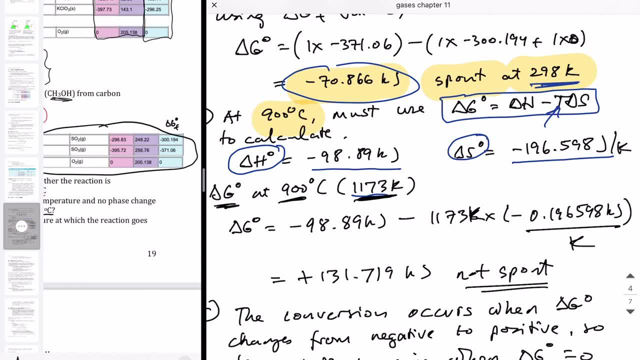 celsius or 1173 kelvin. so keeping in mind that when i do these calculations, i have to use kelvin because it has to do with the use of the gas constant later on in order to do some conversion, so having that as my delta h and 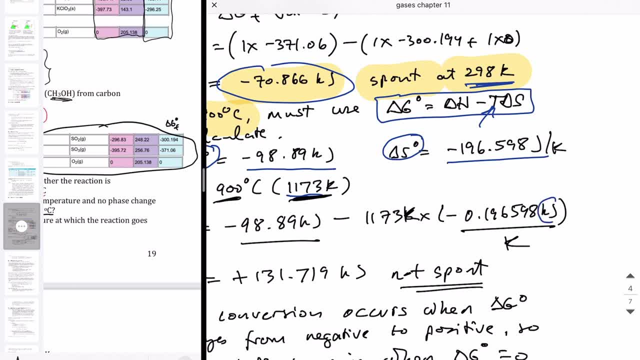 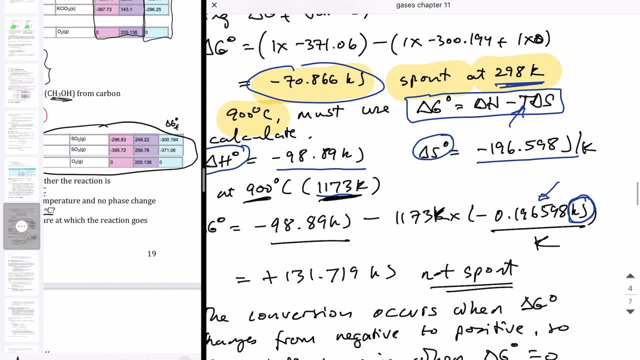 then my delta s remember that i always want to make sure the units are the same. so i convert this to kilojoules, which means dividing by a thousand. so now i have negative point one. nine six, five, nine eight kilojoules per kelvin. so when i apply it in that formula, this is what i get in. 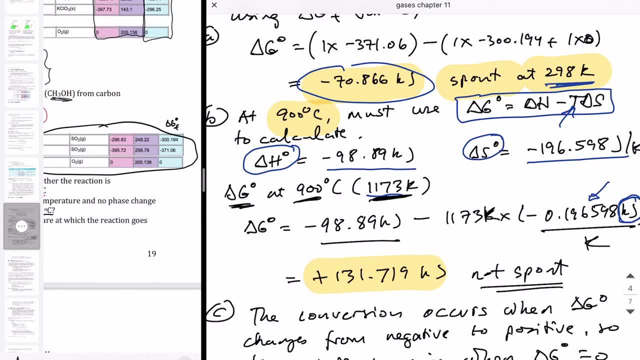 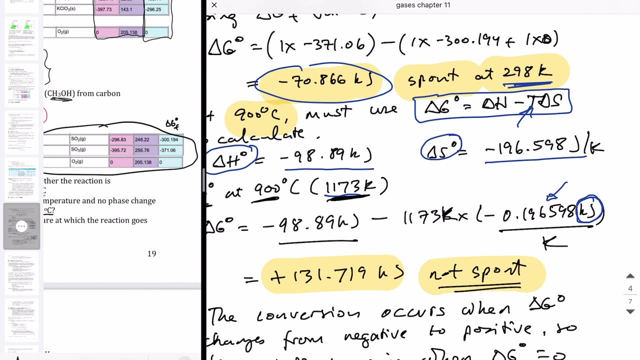 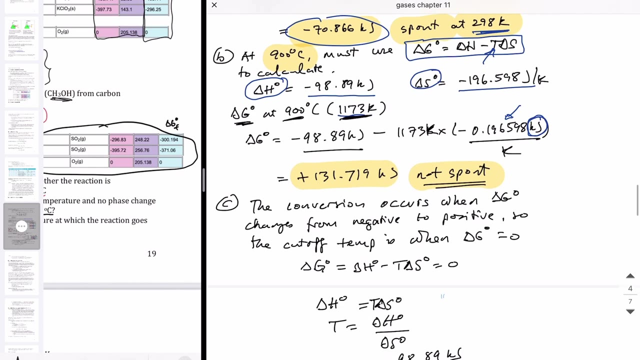 the end, i get a value of delta g standard equal to positive. one thirty one point seven, one nine, four, one, five, zero, three, k. even that's the same number as the one point seven, two, three, zero, one, eight or so, and so, during this process, the average allows us to calculate delta g standard. 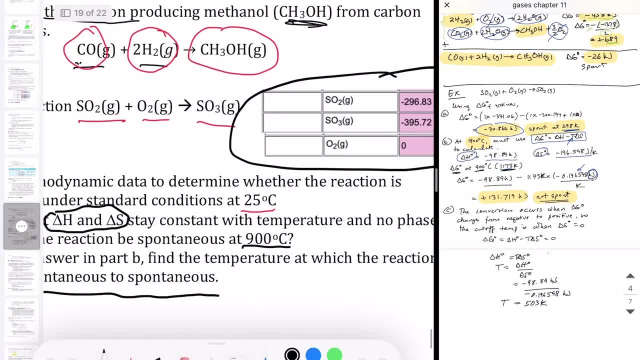 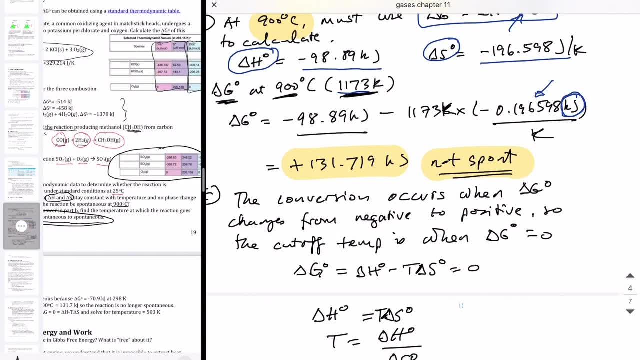 so this is a continuous explanation of the temperature of this Carney for the amount of angelic CO2 applied to a specific energy. so here, in case you have any questions, such as сердечко and a combination of those conditions, we can design a value of delta c c, that is the temperature of. 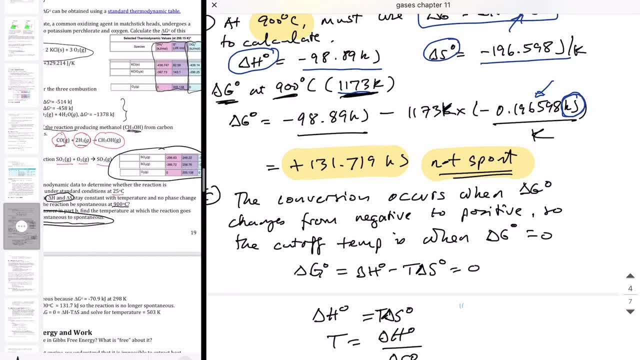 delta G goes from a negative number to a positive number. Well, going from negative to positive requires you to cross through zero. So, in other words, we can find that specific conversion temperature if we set our delta G standard equal to zero, And that's what I'm going to do here. 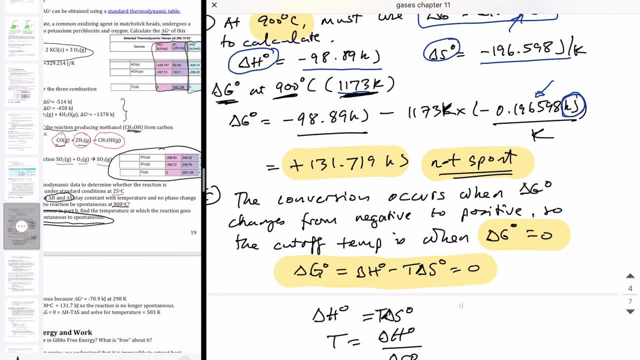 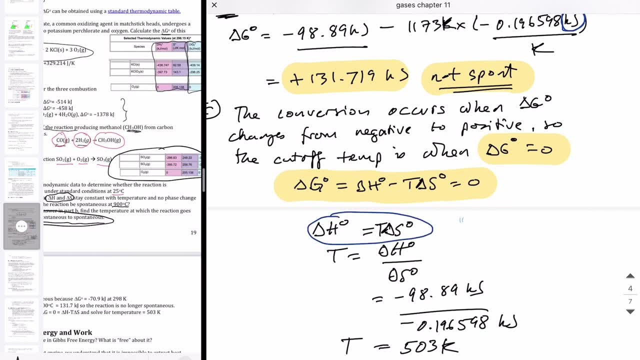 I'm going to say delta G is equal to delta H minus T delta S, but the conversion will happen when that delta G value equals zero. So then that allows you to rearrange the equation and write it this way: delta H equals to T delta S, and then solve for T, which is just equal to delta.